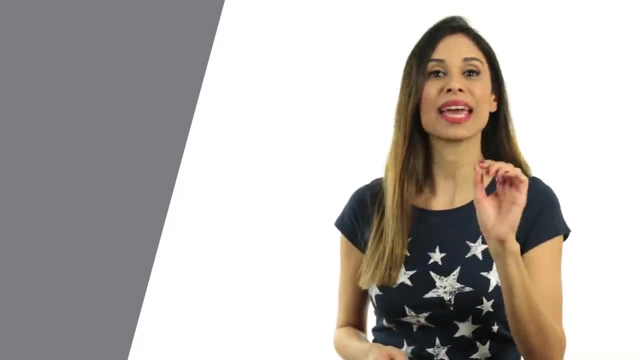 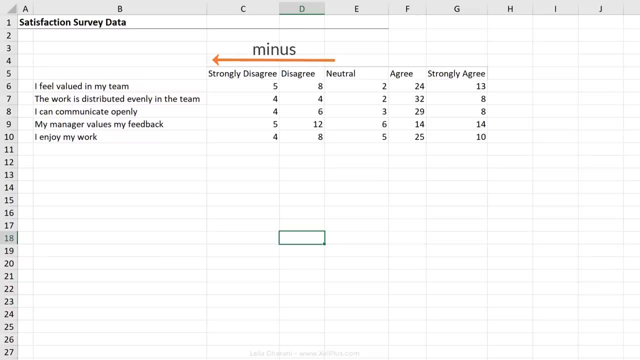 that does it automatically for you without any effort. It's from John, so let's jump in. If you want to get these centered in the middle, we need to have minus values and plus values. Remember that our neutral values split in the middle. 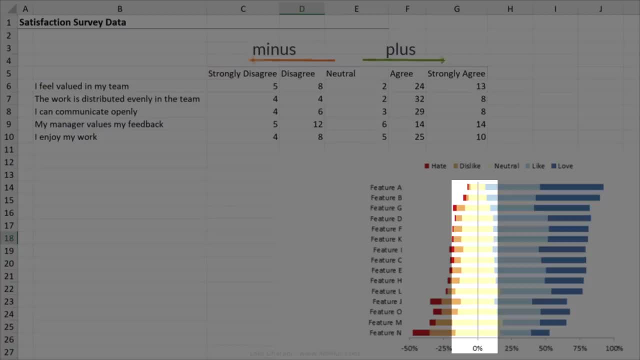 so we actually need to divide those responses by two, and half of them are going to be negative. the other half, positive, Strongly disagree and disagree- are going to be negative for the chart. This means we can't just use this data set. 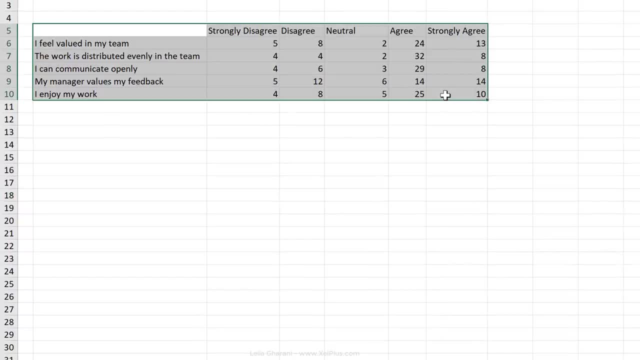 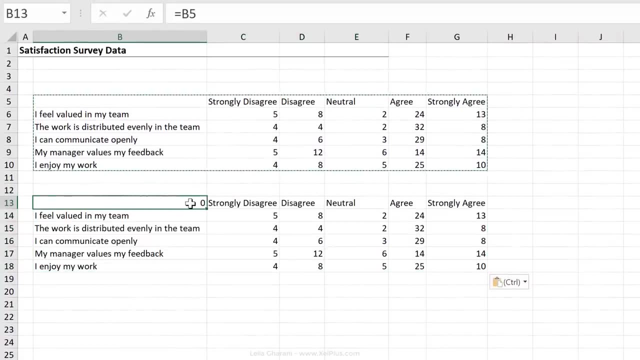 We actually need to create a data preparation table in between. To help us get a head start on that, I'm going to copy paste this here, but I'm going to paste this as links and then tweak what we need to tweak. 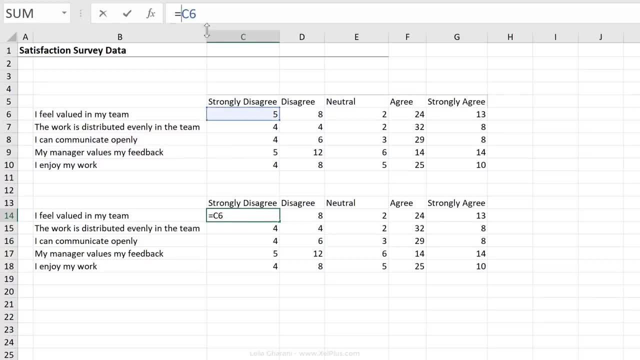 I know that I want to get strongly, disagree and disagree as negative, so I'm just going to put a minus sign in front of the cell reference for these two. push these down. Neutral is something I need to split to two, so I'm going to push them over here. 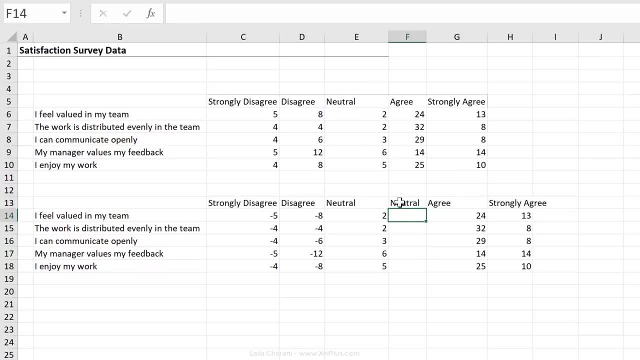 add two neutrals here. One is for the minus side and the other one is the plus side, but I also need them as minus here. so minus the value divided by two. I'm going to push this down. The other one is on the positive side. 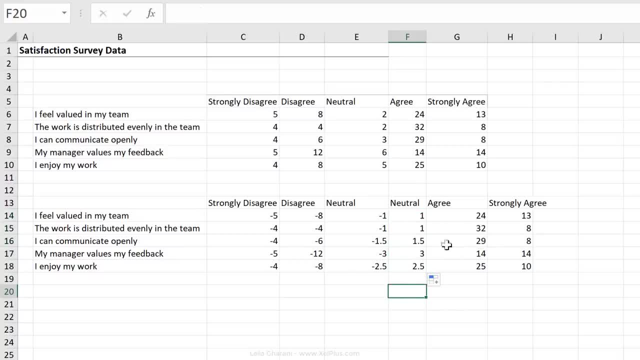 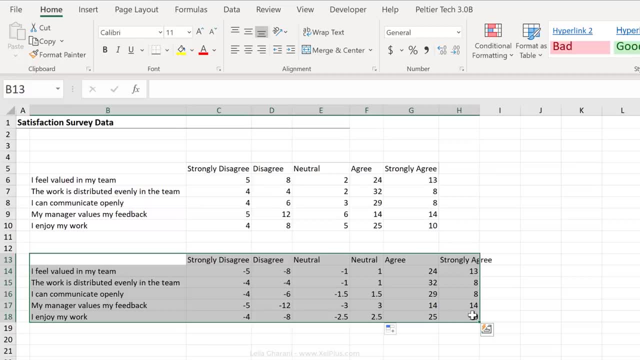 value divided by two. Okay, so this looks good. I'm not exactly sure about the order of the stacks, how Excel is going to stack them, but it doesn't matter. We can get started and then we can fix things as we go. 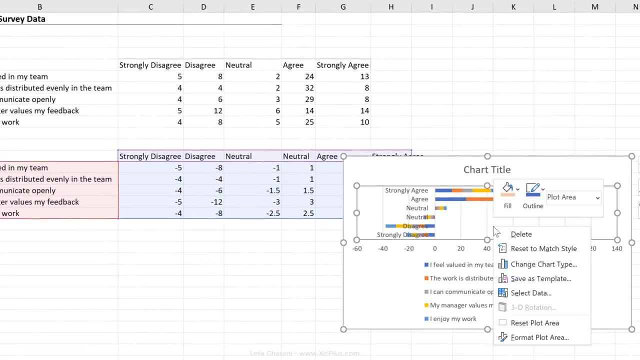 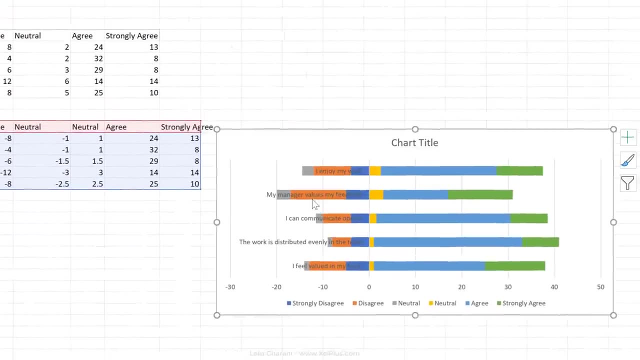 So let's highlight this. insert a stacked bar chart. Let's switch. so select data. switch row and column to get our questions on the correct side. For me to be able to better read this, let's put the labels on this side. 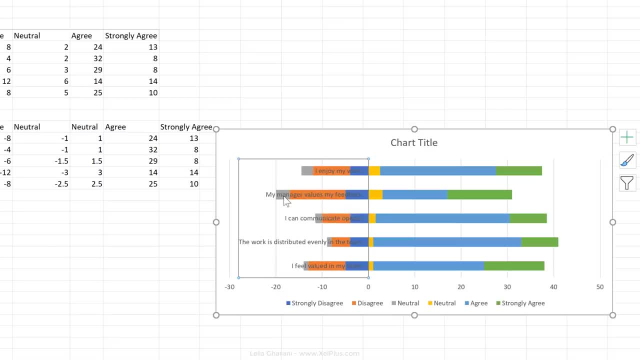 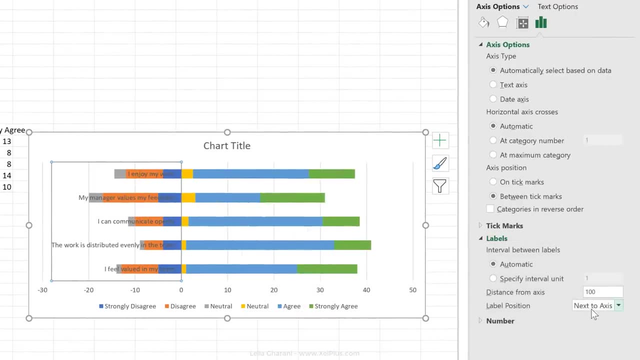 because currently they're covering the minus value. So I'm going to highlight the axis. press Control-1 to bring up the properties Under axis options for labels instead of next to axis. we need low. Okay, so that pushes them. 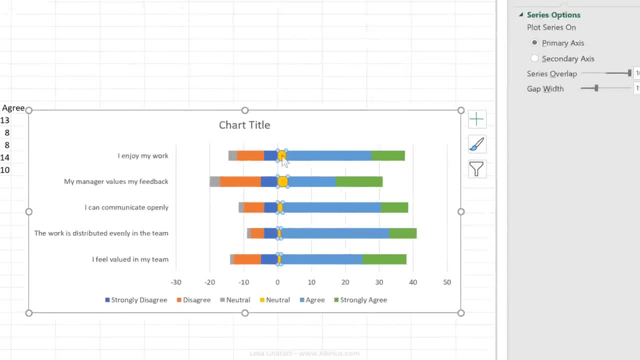 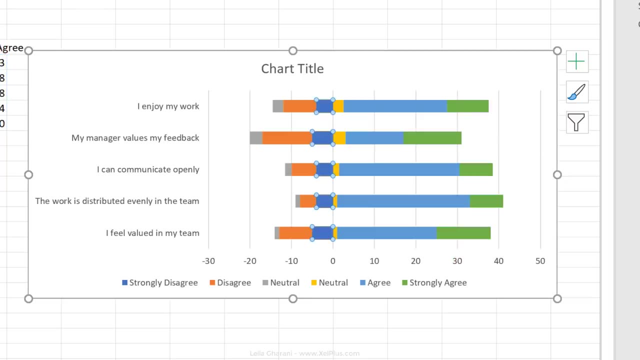 Okay, so that pushes them. Okay, so that pushes them out of the way. Now let's take a look at our stacks. That's the neutral stack. That's the agree and strongly agree. They look fine. This one, that's strongly disagree. 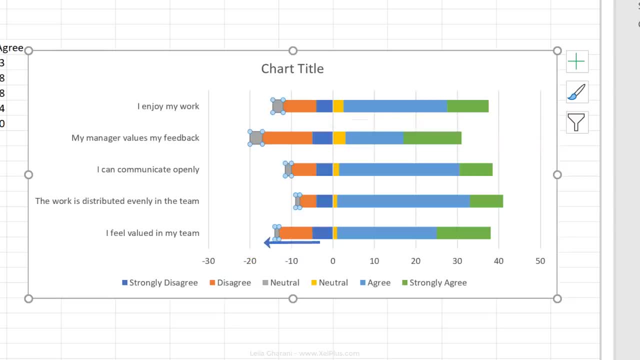 I don't want that here. I want that all the way at the end. This one is neutral. I want it to be stuck to the other neutral right, Because now for neutral, I get two different colors, because I have two different series. 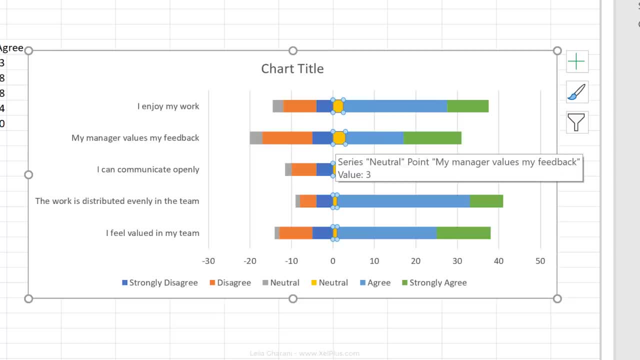 Ultimately, I'm going to make them the same color. They're going to look like one series. They're going to look like one series. but for me to be able to do that, I want to bring this neutral beside the axis, which means I need to switch the position. 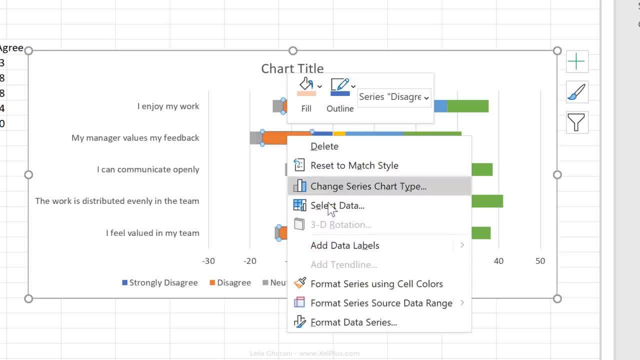 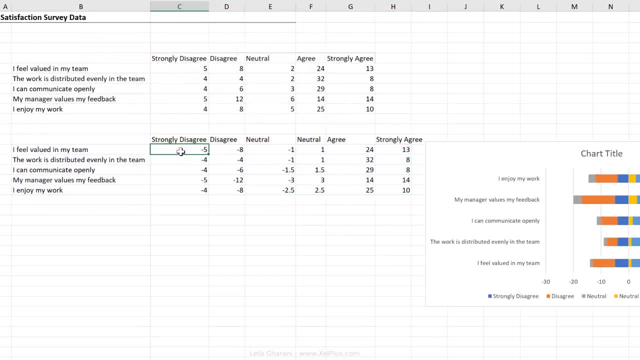 of these two with one another. Now, there are different ways of doing this. I could right mouse click, go to select data and switch the positions in here, or I can do it in my data preparation table. Now, whenever I can, I try to fix things. 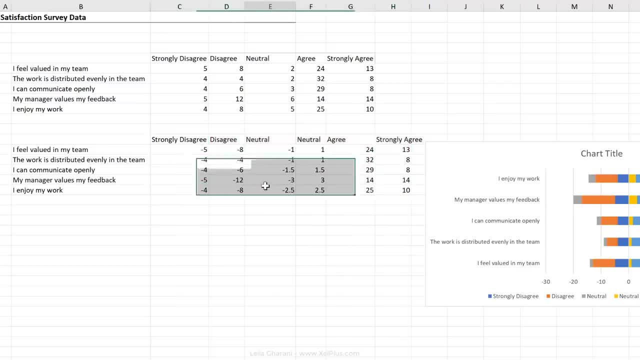 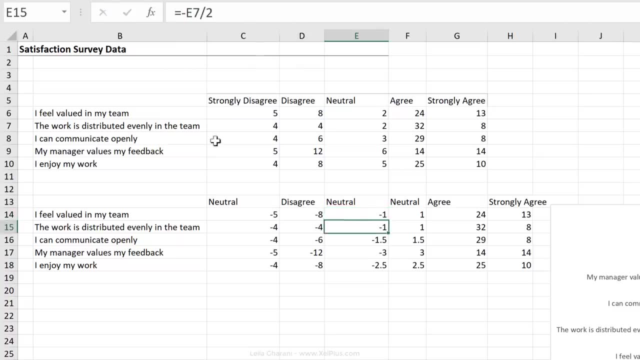 in the data preparation table to keep my chart formatting simpler. So let's just fix it here. This means my neutral category is. This means my neutral category is going to come here and my values here. I'm going to push it here. 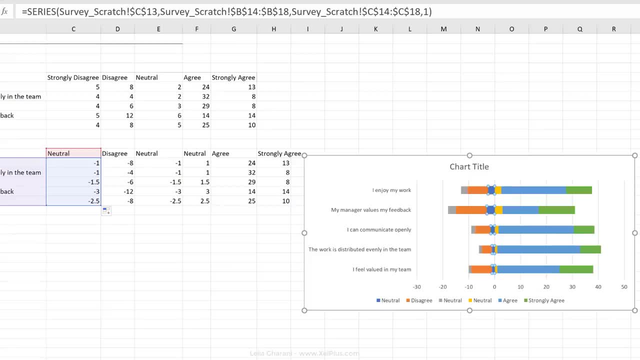 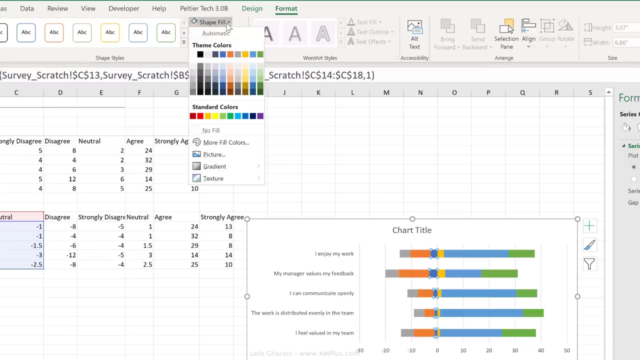 Okay, so now we can see the neutral category shifted to the axis. Let's bring back my strongly disagree. Okay, so now this looks good. Strongly disagrees at the end, then disagree and neutral. Now let's take a look at fixing the colors here. 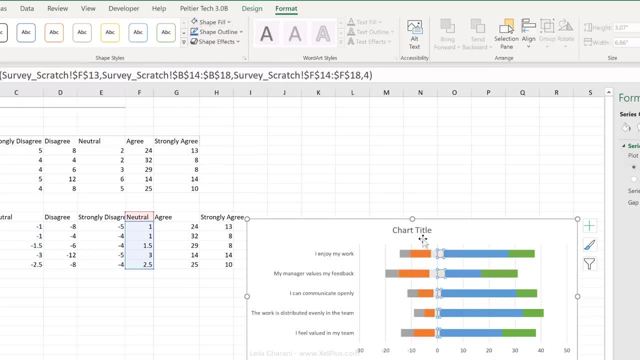 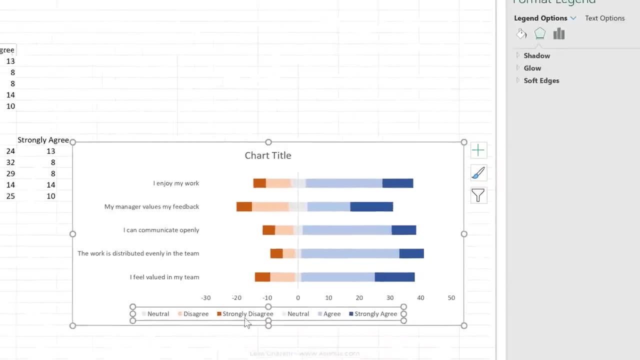 For neutral, I'm going to go with a light gray. This is going to get the same color. Okay, so this looks good. Let's take away the grid lines from this. Let's take a look at the legend. First off, I'm going to push it to the top. 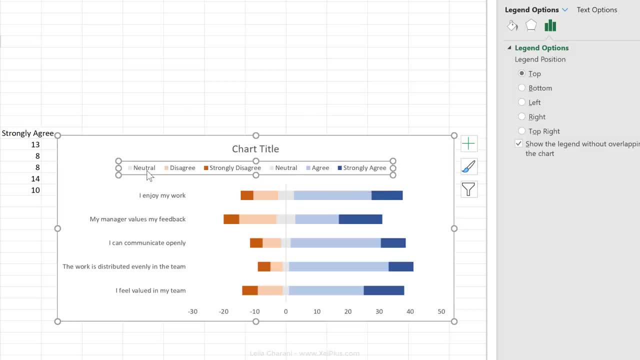 instead of the bottom. I have neutral two times. I just need it once. Click on it two times to only highlight this and press delete. Now what I don't like is the fact that disagree comes first and then strongly disagree. 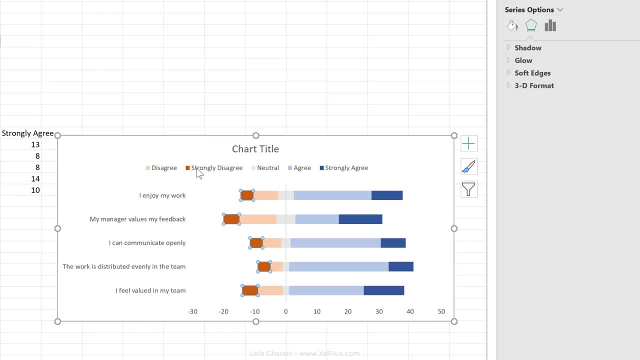 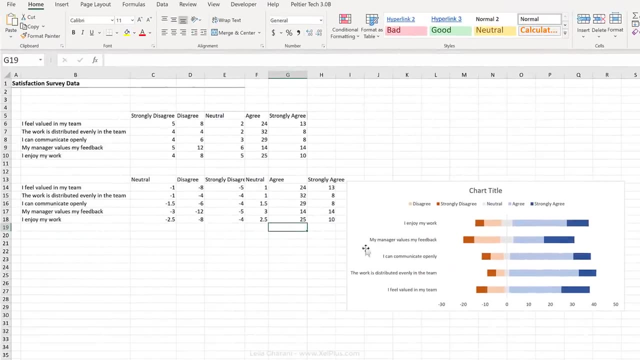 Whereas on the chart I have them in the correct order, The legend is not correct, So before we take a look at how we can fix this, let me show you John's utility that helps us get this done without us needing to worry about our data preparation table. 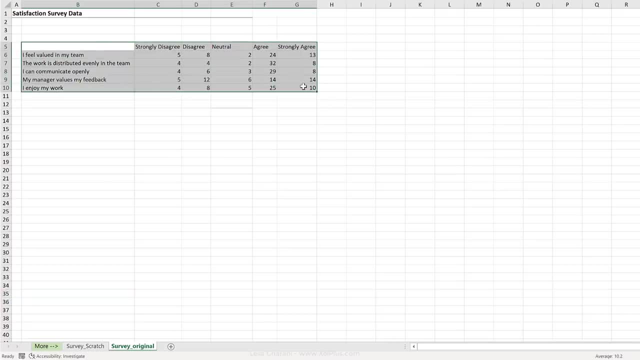 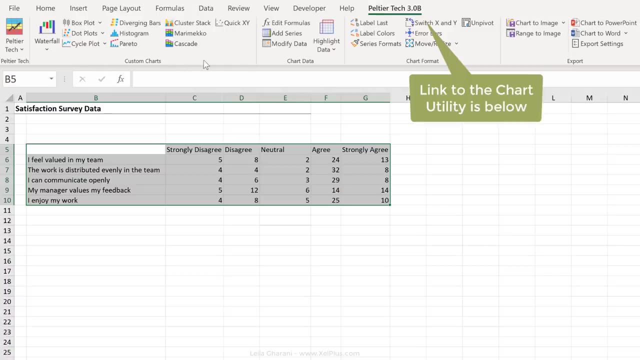 So I have the original data set here. All I'm going to do is to highlight this. Go to Peltier text. so this is the add-in from John. You get a lot of different functionalities here, So a lot of difficult charts in Excel. 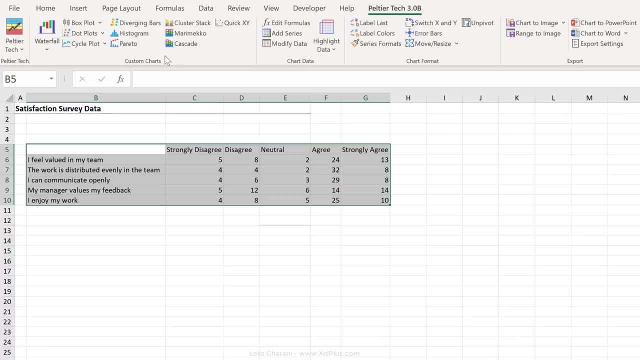 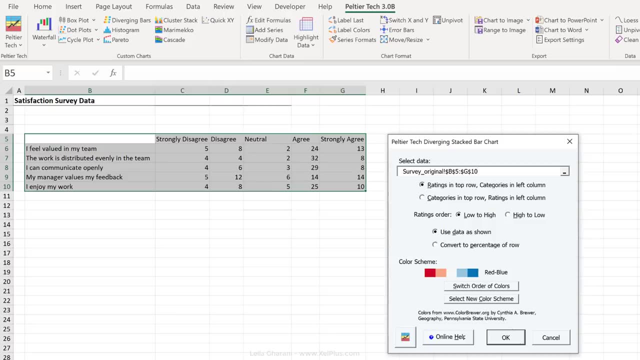 that take a lot of data preparation are made automatically by this tool. Okay, just like what we did, which is called the diverging bars. So I'm just going to click on this, Going to go with the default, not going to worry about colors or anything. 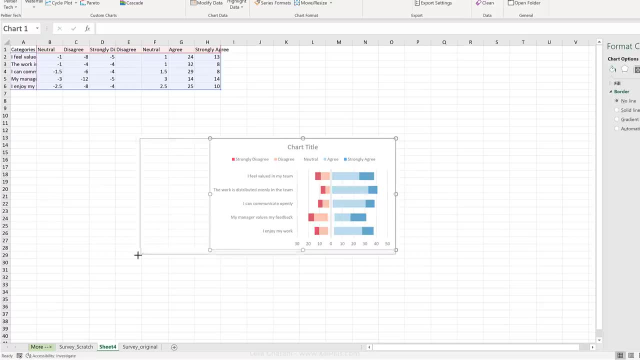 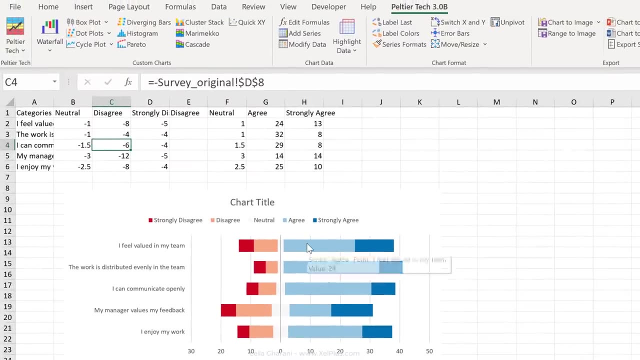 It creates a new sheet for me with my data preparation table, So it did that on the fly for me. It's all linked to the original data set and it gave me the chart and it gave it to me in the right order. 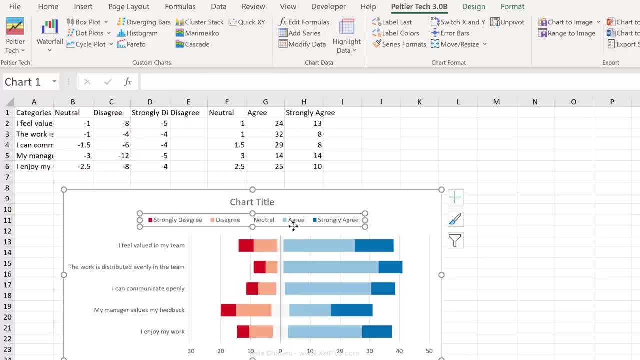 So strongly disagrees here, then it's disagree, neutral, agree and so on. And this is a normal chart, so you can change these colors just like you can do any other chart. So this is a normal chart, so you can change these colors just like you can do any other chart. 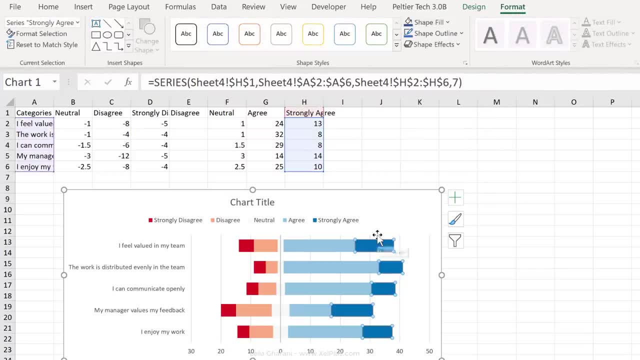 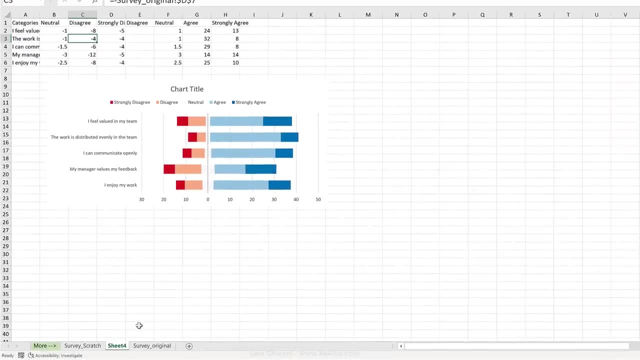 So this is a normal chart, so you can change these colors just like you can do any other chart. One of the great things I like about this is that it doesn't hide the work from you. It shows you the data preparation table. It links it to the original data set. 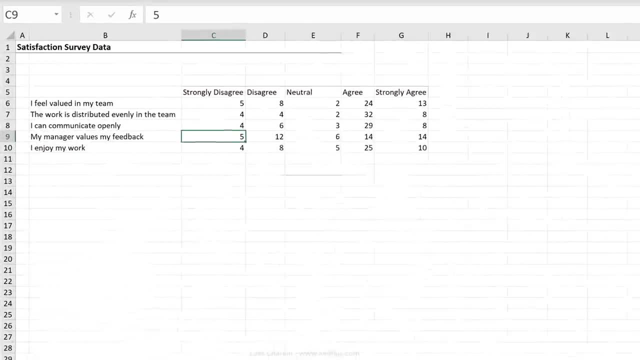 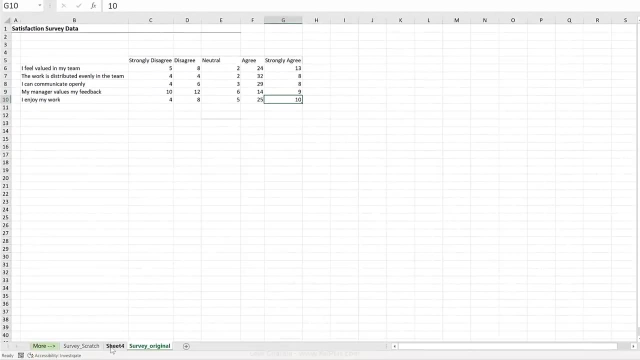 We can actually test this quickly. Go to the survey results. Here I have five people. Let's change it to 10.. Let's change this to nine. Okay, let's go back here. We can see: this got bigger, this got smaller. 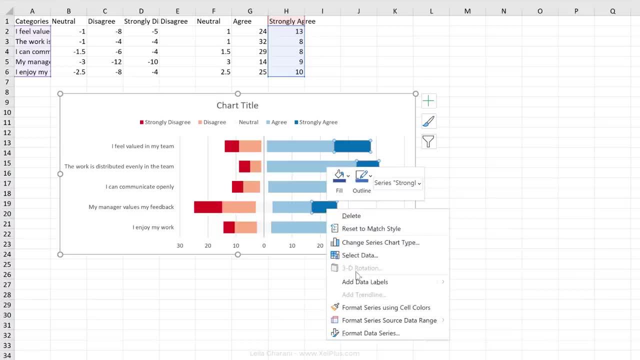 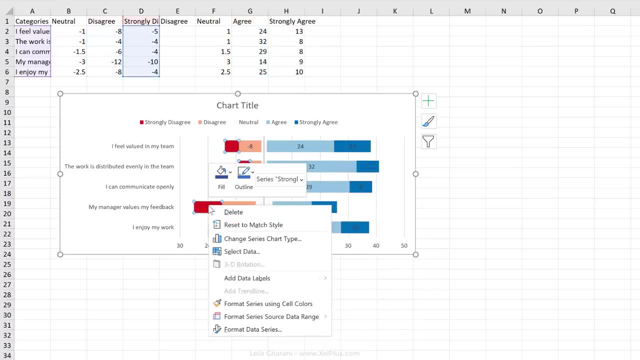 Now, one thing you might want to do with this chart is to add data labels, And you can do that really fast: Just right mouse click, add data labels And neutral one. I'm just going to leave out the labels. I'm going to add them here as well. 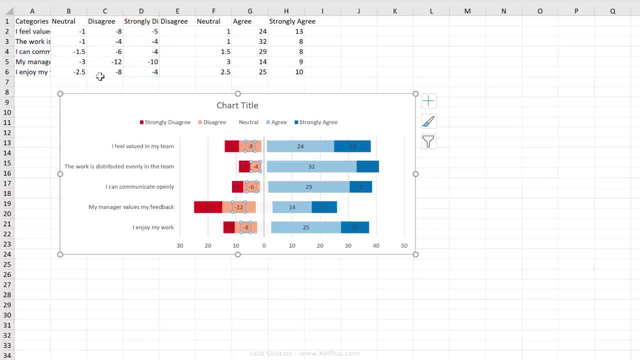 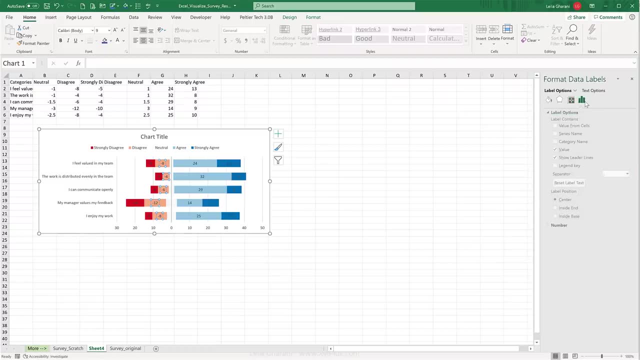 But I don't want to show minus people, right? I actually want to show these negative numbers as positive numbers. This is where I can use custom number formatting. So from the formatting options here for number, I'm going to give my own format. 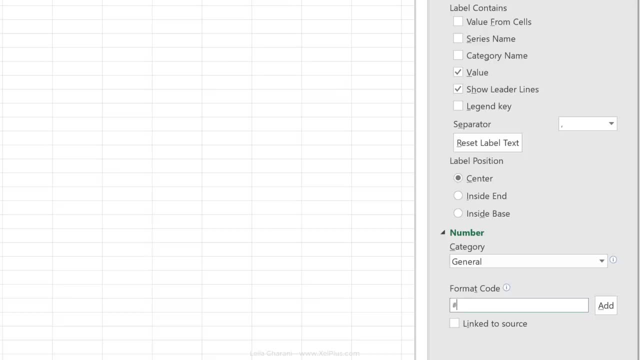 and I'm going to say: well, positive numbers should be formatted as a positive. So the hash sign is just a placeholder for number. I'm not going to use a thousand separator in this case. The second argument is how negative numbers should be formatted. 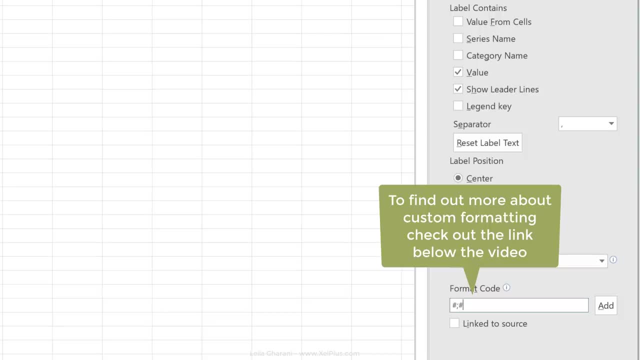 And if I omit the negative sign from this, they're going to be shown as positive, right? So remember, custom number formatting has four arguments: First is positive, then is negative, then is zero and then is text. I just need positive and negative here. 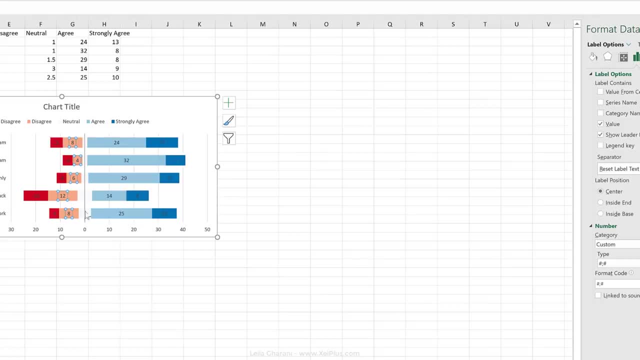 And I'm going to add a hash sign for both, so that my negative numbers look like positive numbers. I'm going to do the same for this, So that's easier to read the data. You can change the color of the labels and we can delete this. 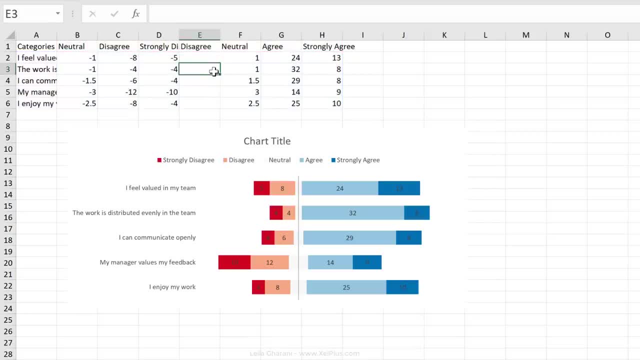 Now remember what I said before, that what I like about this is it doesn't hide the work for you. What you can do is learn a lot from this. How did this add-in manage to get strongly disagree first and then disagree? We can see it from the data preparation table. 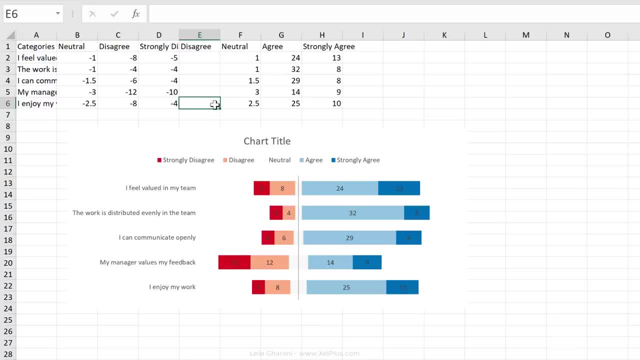 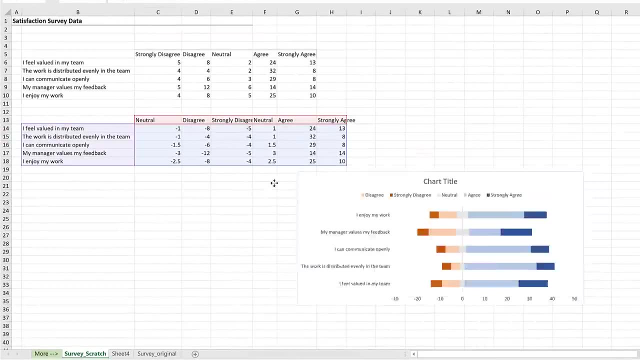 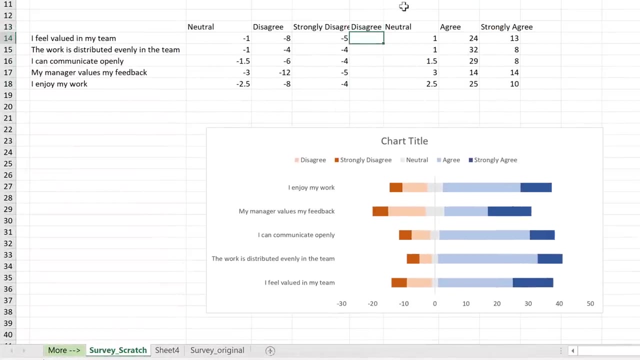 Notice we have an extra disagree column that we didn't have in our data preparation table. Well, the purpose of this is purely for the legend. Let's go back to our data preparation table, shift these out of the way, add a dummy disagree series that has no numbers. 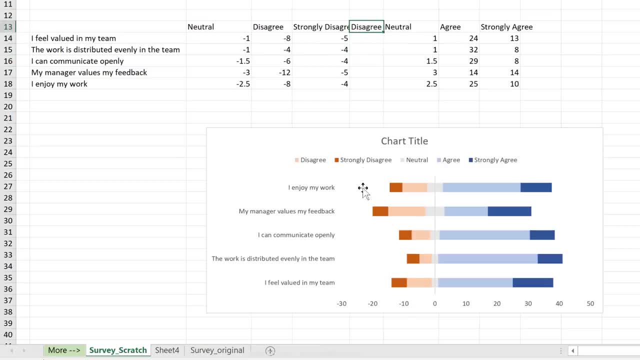 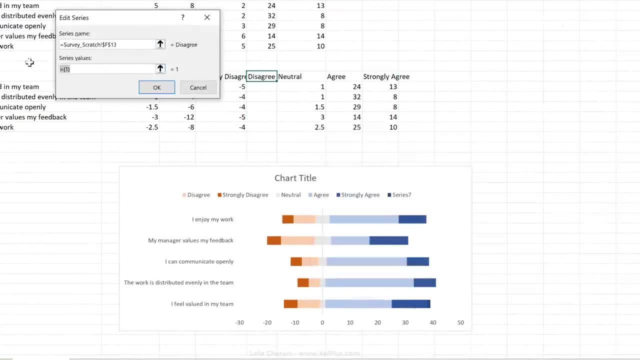 The pure purpose of this is to get the legend correct. So now I'm going to add this new series to my chart. Select data: add For series name. it's disagree Series numbers. They're just going to be these. They're going to be empty. 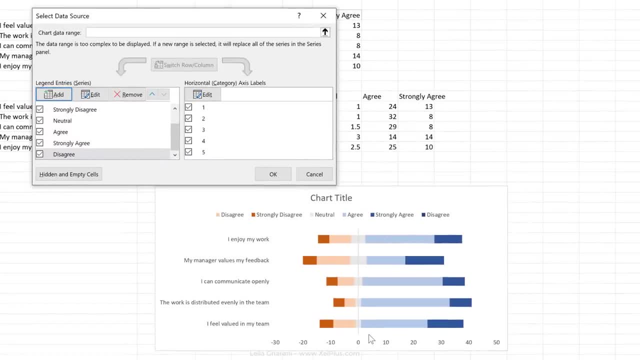 I get a new legend. It has no numbers. I can't see the series here Now. I'm going to push it where I want. So notice, when I push this up, it moves in the chart as well. I'm going to position this right where I want. 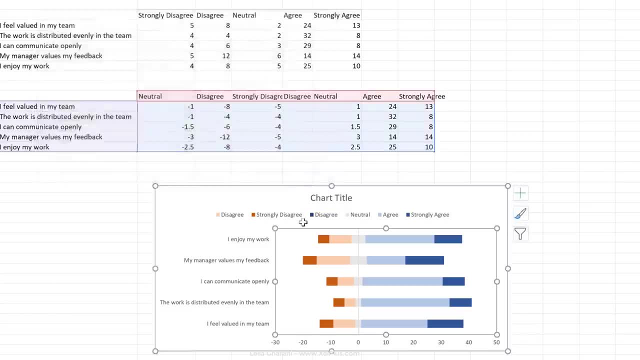 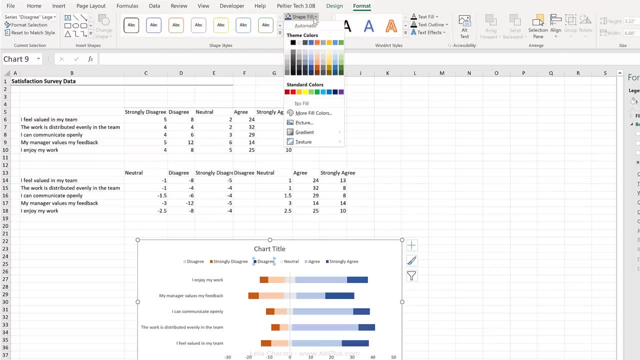 I want it after strongly disagree, So I'm going to go with: okay, I'll click on it, click on it again, just to select this and go to format and change the color to the disagree series. right, Because I want this to be identical to this. 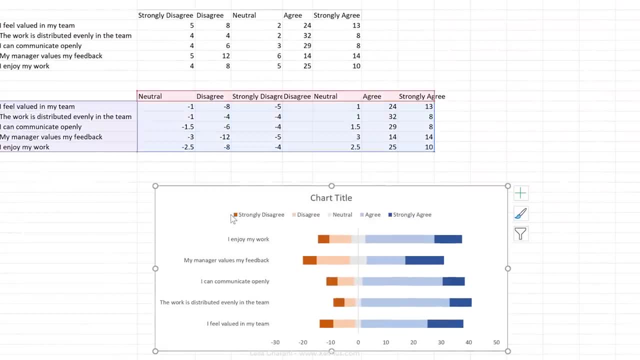 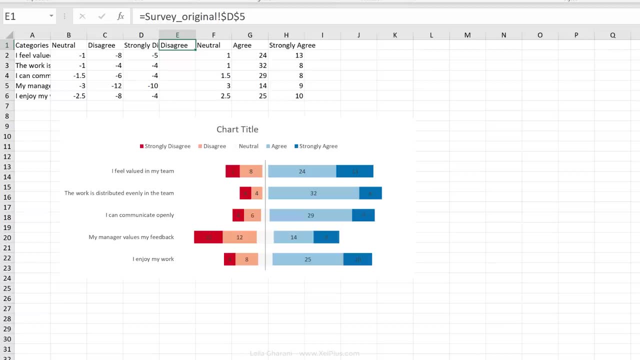 I'm going to delete this click click and then remove this from view right. So the great thing about John's utility is not only that it does the work for you, but it allows you to learn from it, because it doesn't hide the data preparation from you. 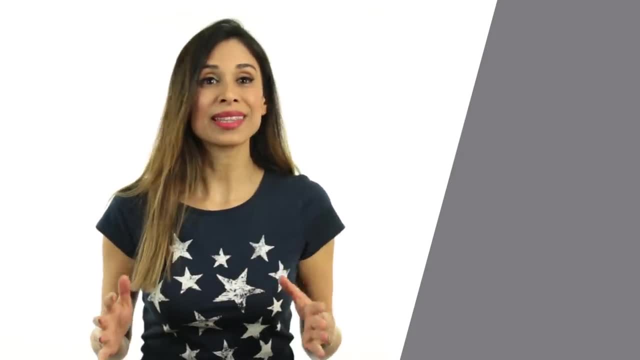 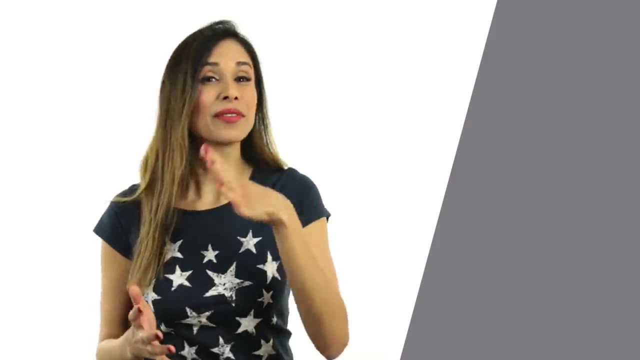 I've added the link to the description of this video. Please note that this is not an affiliate link. If you follow my tutorials, you know I'm a big fan of advanced chart techniques. I'm a big fan of advanced chart techniques. I'm a big fan of advanced chart techniques in Excel from scratch.